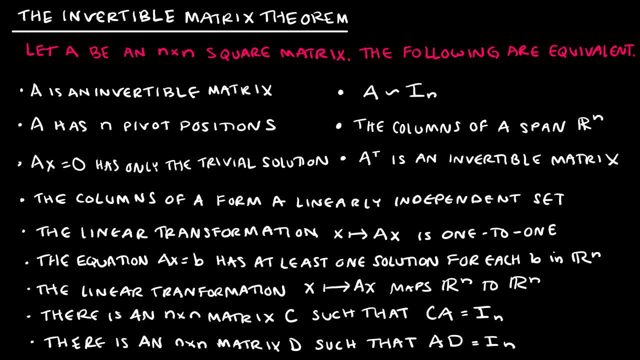 a great job of summarizing pretty much everything that you learned in chapter 1 and everything that you've learned in chapter 2.. Specifically, though, for an n by n square matrix. So yes, when we worked on matrices in chapter 1 and some of chapter 2, they weren't. 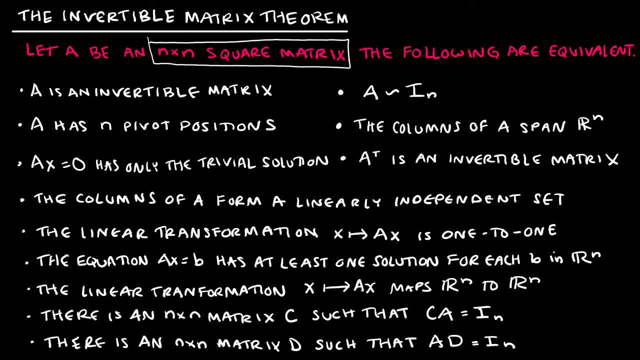 always square. but those concepts that we learned all can be applied to these square matrices, And what the invertible matrix theorem says is that everything in this list is equivalent. What that means to you is if you can show, for instance, that a row reduces to the identity. 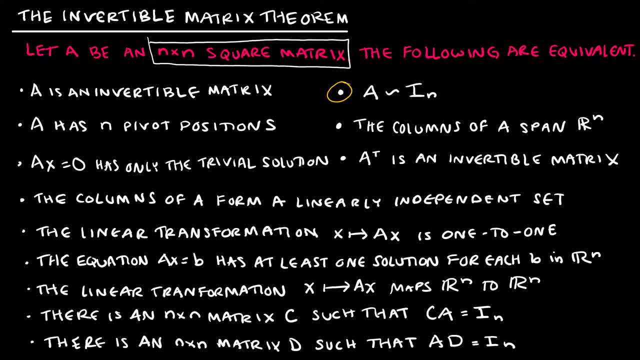 matrix. Then you can say: everything else on this list is also true about a. If you can find that a does not have n pivot positions, but in fact has fewer than n pivot positions, then you can say that everything else on this list is false. So everything that is. 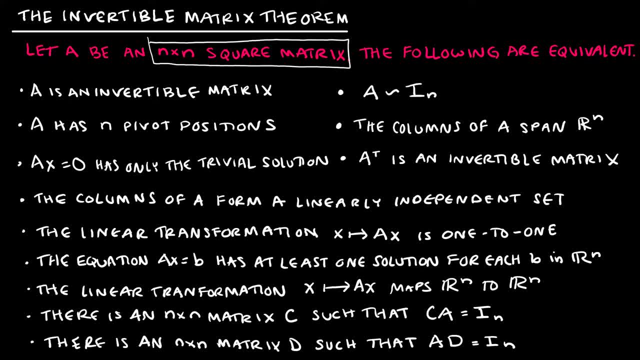 listed here for the invertible matrix theorem. all of those statements are equivalent statements. A is invertible, A row reduces to the identity matrix. A has n pivot positions. The columns of A span, Rn, Ax, equals 0, has only the trivial solution. 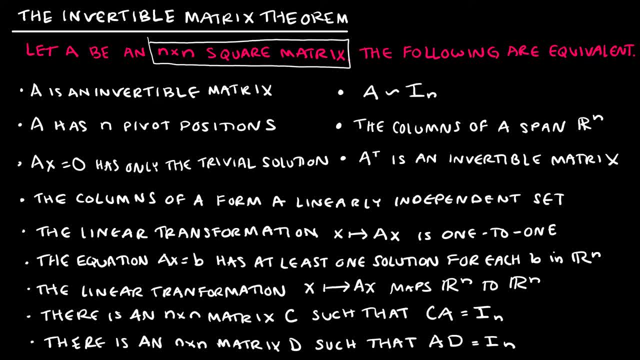 The transpose of A is an invertible matrix. The columns of A form a linearly independent set. The linear transformation that maps x to Ax is 1 to 1.. The equation Ax equals b has at least one solution for each b in Rn. 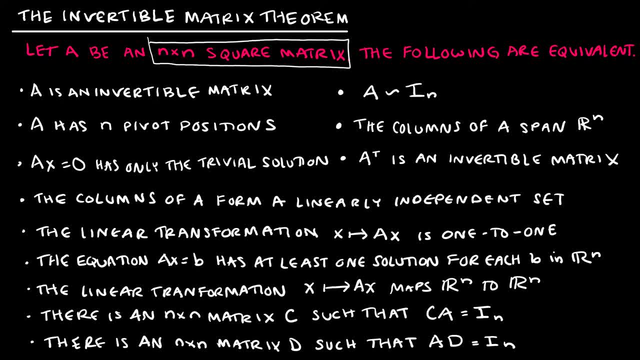 The linear transformation that maps x to Ax, maps x to Ax to 1 to 1.. So everything here happens: when you substitute Rn with Rn, There is an n by n matrix C, such that C equals the identity, and there is an n by n matrix D, such that A times D is equal to the identity. 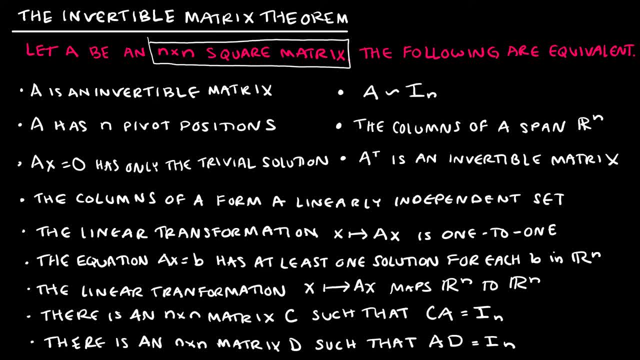 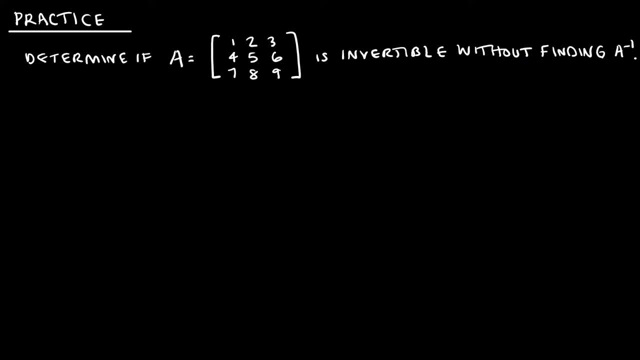 All of these things mean the same thing. There's really not a whole lot of need for practice, because really that last slide just summarized things that you already knew, so this is not anything new. but let's go ahead and look at other materials for practice alone. There's really not a whole lot of need for practice, because really that last slide just summarized things that you already knew, So this is not anything new, but let's go ahead and look at one of my other good examples here. So let's forget about all of this. 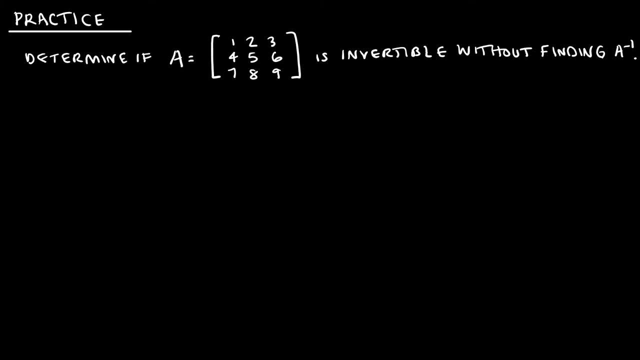 This is bringenism ahead just for fun and do a couple of practice questions. so this first one says: determine if a is invertible without actually finding the inverse. so if I had to find the inverse, I would write down a and then I would augment it and to the right I would put the identity. they're saying: don't bother. 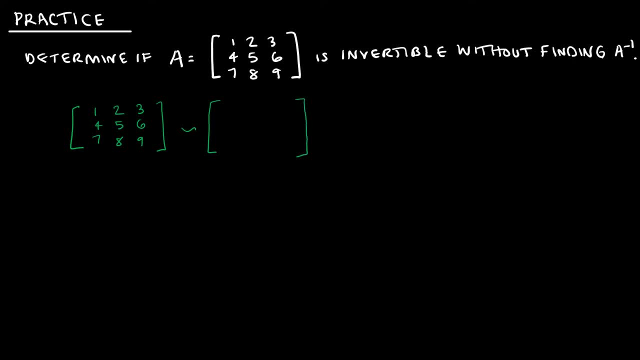 just do your row operations. so my first row is going to remain the same and my second row I'm going to take negative 4 times my first row and add it to row 2. so negative 4 plus 4 is 0. negative 8 plus 5 is negative 3 and negative 12. 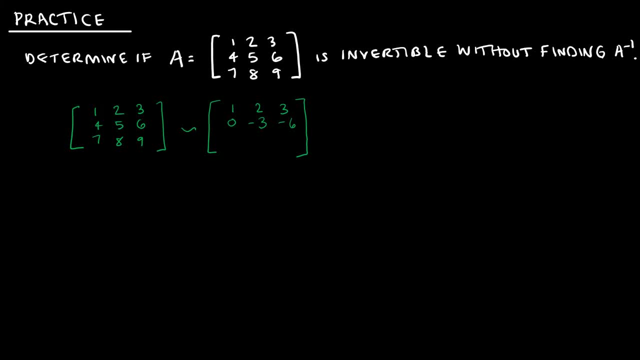 plus 6 is negative 6, and then I'll do the same, but with negative 7 times the first row, which gives me negative 7 plus 7 is 0. negative 14 plus 8 is negative 6 and negative 21 plus 9 is negative 12. next thing I'm going to do: 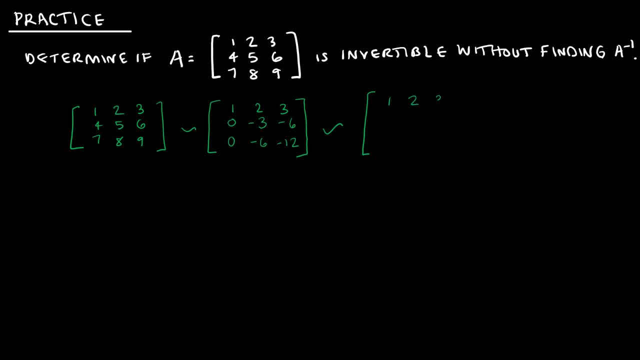 you. you is, of course, keep my first row the same, My second row and my third row. obviously, I'm seeing what's happening already, but let's go ahead and finish. I'm going to take my second row, times negative one-thirds and that's going to give me one and two. so I've got my pivot here and pivot. 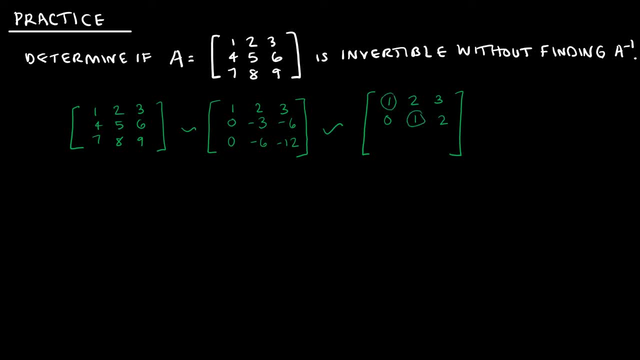 here, and when I take my second row, times negative two to add to negative three, I end up with zeros here. So what I have found is that I do not have a pivot in every row, so we cannot find a inverse since there is not. 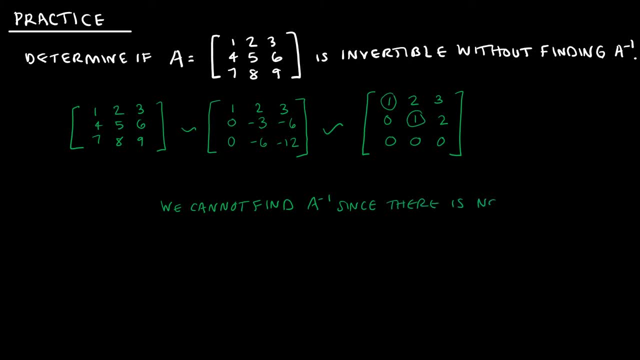 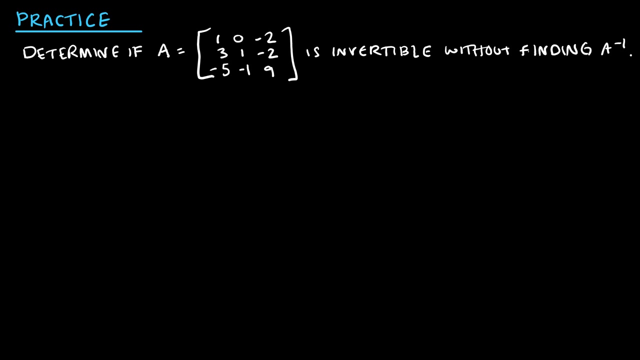 a pivot in every row, And then that's, of course, by the invertible matrix theorem. As always, here's one for you to try. so press pause, try this question, then press play to see how you did So. again, I'm just going to take A.